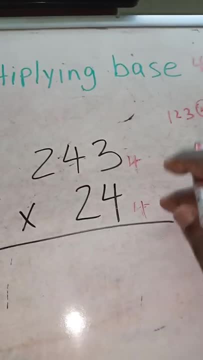 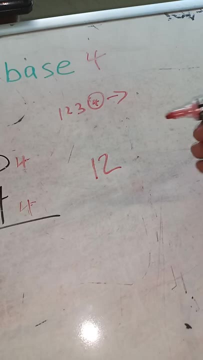 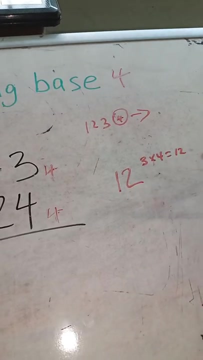 okay, you never. you can never write a number the same value as the base number. all right, has to be lower. let's jump right into it before. three is equal twelve. you can't write twelve three times four equal twelve. so we see that four can go into twelve three times and the remainder would be: 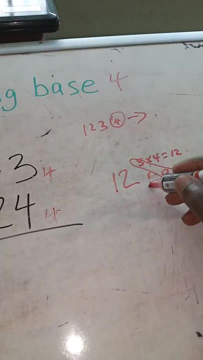 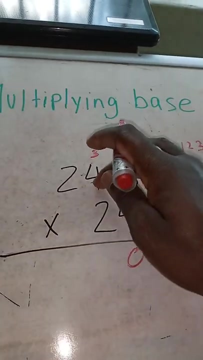 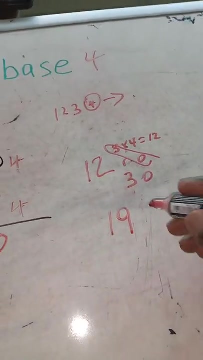 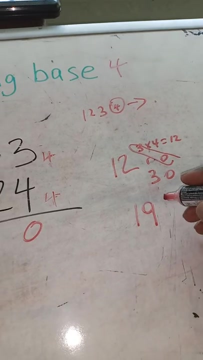 zero. all right, so the representation for four would be three, zero. what do we do with the zero? put it down and we carry the three, all right. four, four, sixteen, seventeen, eighteen, nineteen, four, four, sixteen and three equal nineteen. although we write nineteen three times four equal twelve. four four equals sixteen, right, so four times four equals. 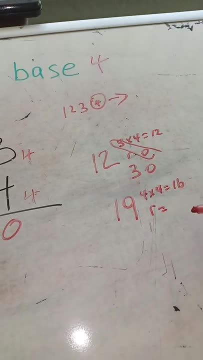 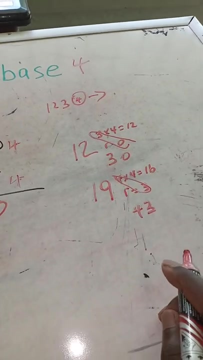 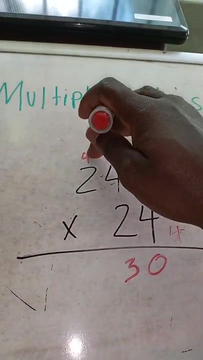 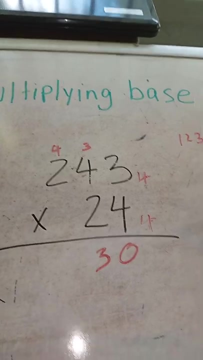 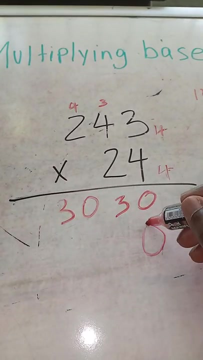 sixteen and the remainder would be what? three? all right, so four, three would be the way we write, nineteen. so we put down the three and we carry the four. four, two is eight and four equals twelve. all right, and we say we write twelve as three and zero. so we put it all down here. then we had a zero. 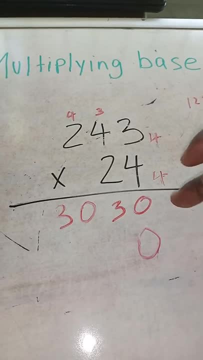 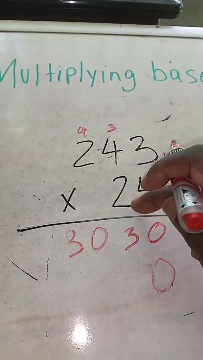 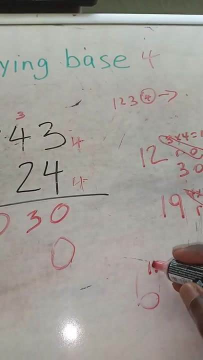 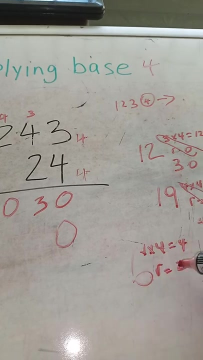 here, because this is a ones column, this is a tens column, so you have to have a zero. is one zero on ten? so you put one zero here. okay, good, two times three equal six. can we write six in base four? no, but one times four equals four, remainder equal two. so one, two would be the way we write six in base. 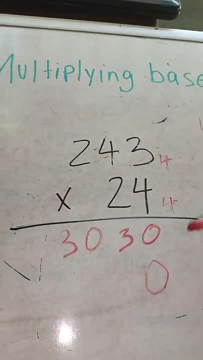 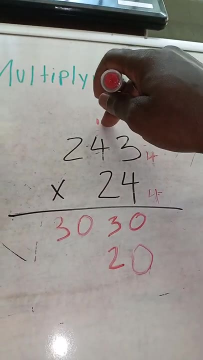 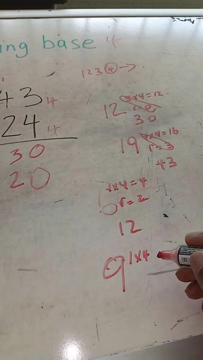 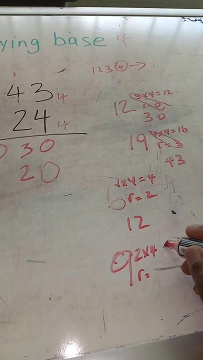 four. all right. so what do we do now? we put down the two charlie, one, two, fours eight and one, nine. although we write nine in base, four of the times, four can go into nine one times and remainder is equal to what. now we can go in two times two. fours eight equals eight and the 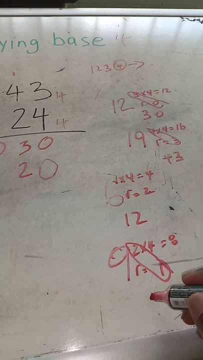 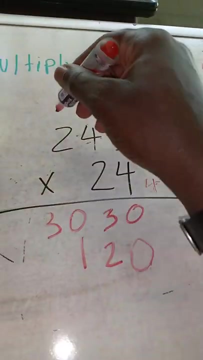 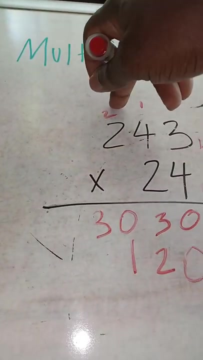 remainder is one, so two. one is the way we would write for nine. so we put down the one and we carry the two. two, twos four plus two equals six. two, twos four plus two equals six. this is the way we write six in base: two, a one and a two. 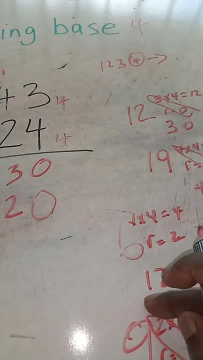 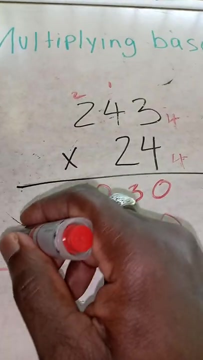 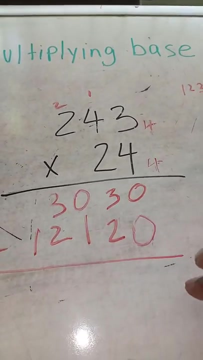 2, 1, 4 and remainder is 2, 4 plus 2 equal 6. all right, so we put down 12 right there. then we're going to do our addition factor factor: equal product, partial product, partial product. let's add the two partial product to get our final product: 0, 0, 0, 3 and 2 equal 5. can we write 5? 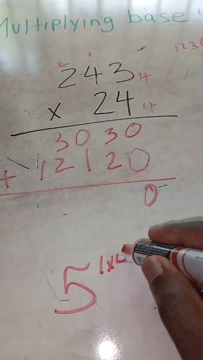 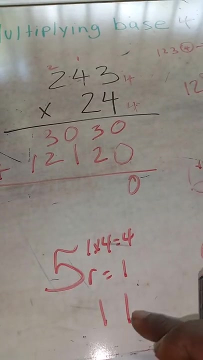 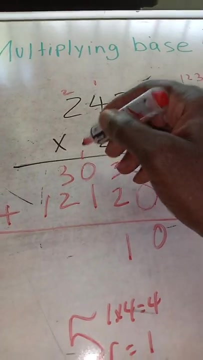 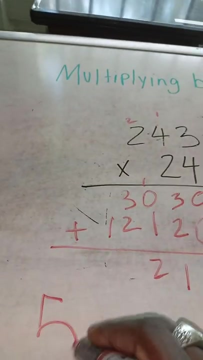 in base 4, no 5 is what: 1 times 4 equal 4, remainder equal 1. 1. 1. 4 plus 1 equal 5. 4 plus 1 equal 5. so we put 1, 1, 1 plus 1 equal 2. we can write 2, 3 and 2 equal 5. can we write 5 in base 2? 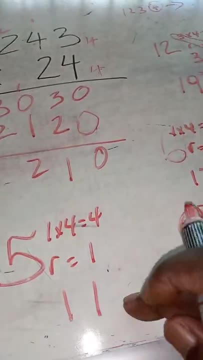 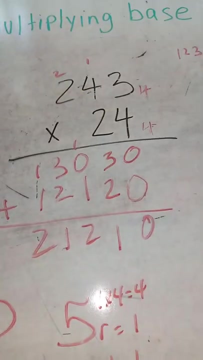 no, and remember we just did a while ago: 1 1 1 1 1 1 1 equal 2. all right, so that is all. we can multiply using base 4. 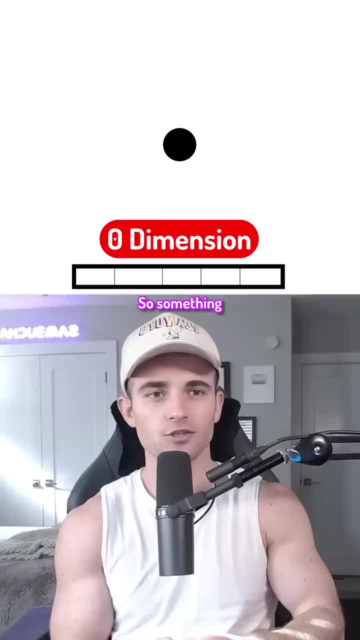 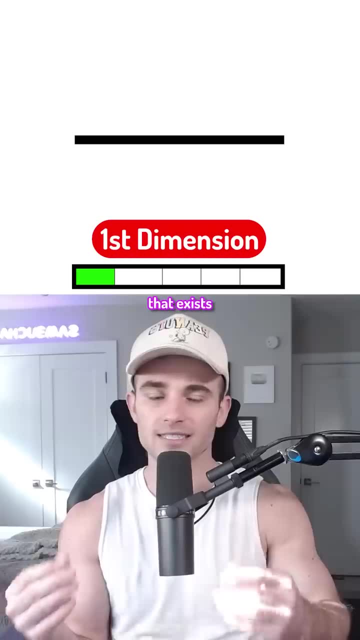 I'm about to show you the fifth dimension, so get ready. So something with zero dimensions you can think of as a single point. It has no substance to it. A one-dimensional object would be a line that exists only in terms of length and has no other. 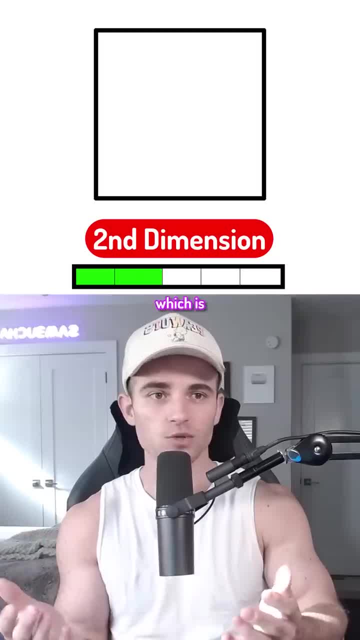 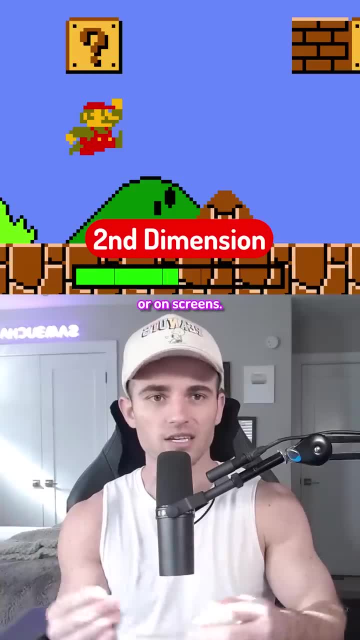 discernible qualities. Add in height or a y-axis, which is another objective quality, to an object and you can see the second dimension. This is generally what we see on paper or on screens. The third dimension adds in depth, therefore now giving an item volume like a cube. 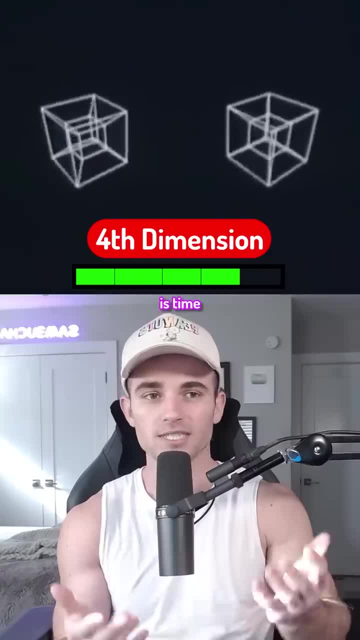 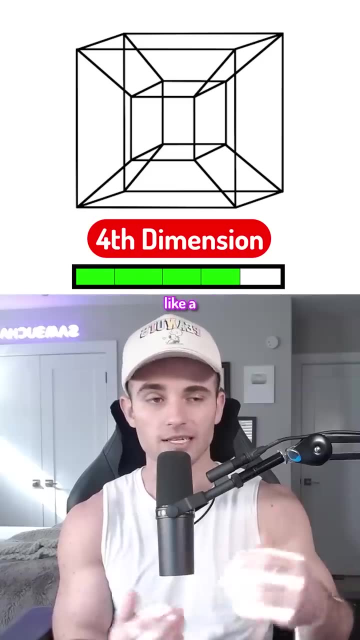 This is where we live, our spatial reality. The fourth dimension is time, and refers to how the three-dimensional objects are positioned in relation to a point in time. Visually, it would look like a tesseract. This is what our reality is: space-time. And so the fifth dimension would: 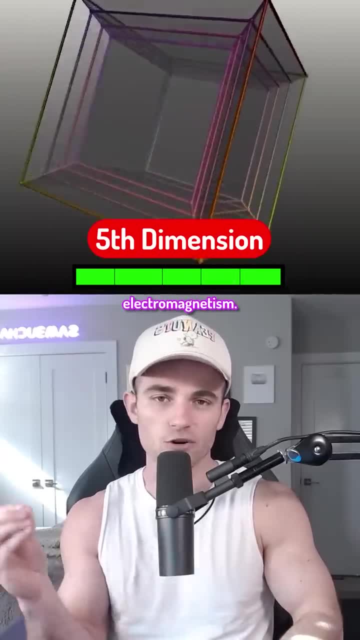 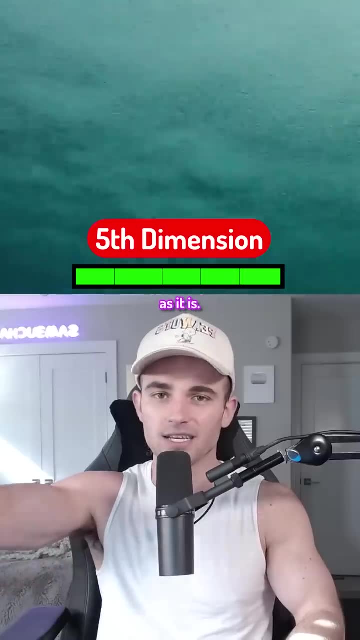 be a micro dimension of space that ties between gravity and electromagnetism. Think of it like when you're underwater and it starts to rain and you see the ripples above. You don't actually see the ripple as it is. instead you see a shadow. That's the easiest way to explain it.